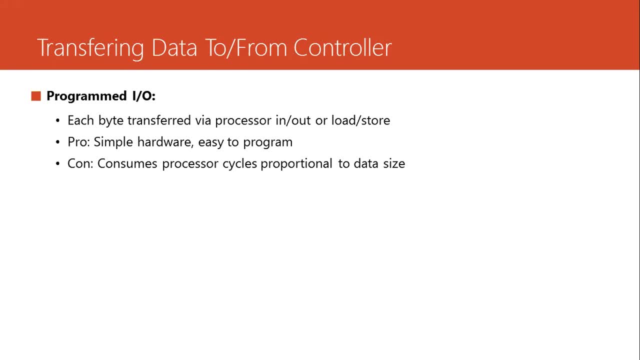 operation, such as the load in the loop, to acquire data from a certain location and not take advantage of a dedicated hardware to do that for you, Right? So this is basically the concept of direct memory access, which requests a device to transfer data directly to the 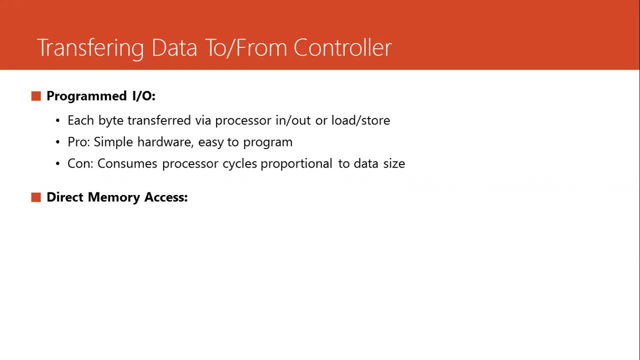 DRAM through the DMA controller. The processor tells the DMA when to transfer the data and how much to send, and then the processor gets out of the loop and the device gets ahead and transfers the data, While the processor only finds out the data out when interrupt from the DMA. for example, the disk drive access works on. 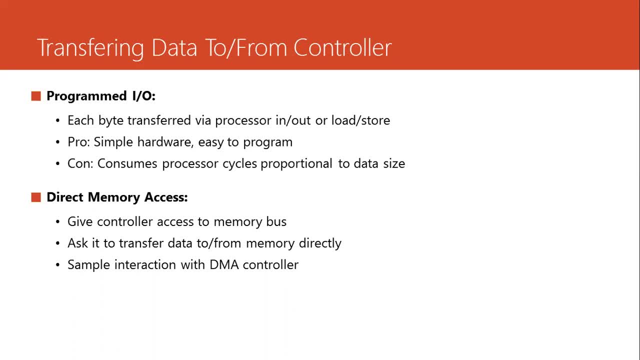 this line, the processor requests a certain number of blocks in a certain location in memory and goes to do other processing and the DMA controller interrupts when the transfer of data is complete. rather than having to wait till it go to that part of the disk and then load a byte at a time and load it to. 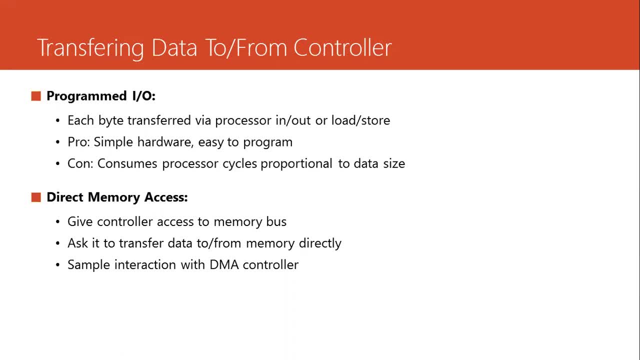 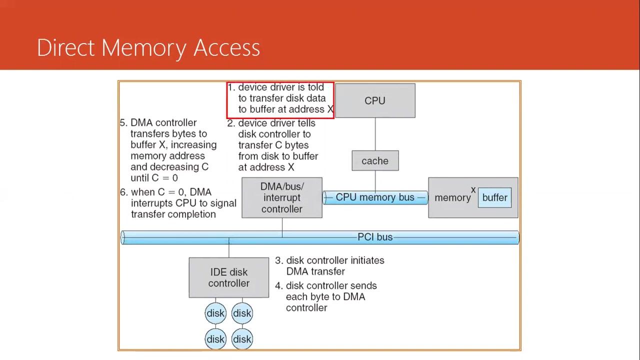 memory. so you can see how much processor cycles were being wasted in the program. right? so the processor asks the DMA controller to transfer data to and from the memory directly. let's see a sample interaction with the DMA controller. the device driver is directed by the processor to request the disk to transfer the data to the buffer, and. 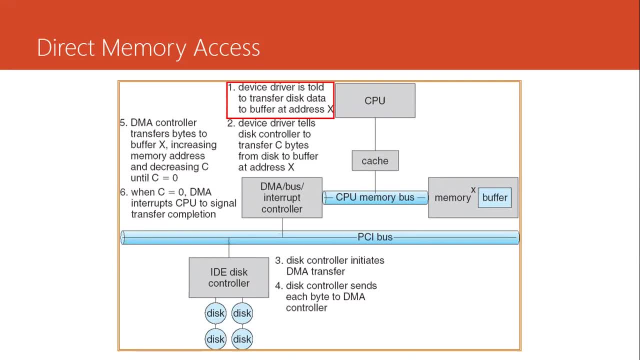 therefore, the processor requests the disk to transfer the data to the buffer at location X in the DRAM. the device driver then goes ahead and programs the disk and the DMA controllers, saying okay, these are the blocks that are required and here is the address of the buffer you should put the data in. and here are: 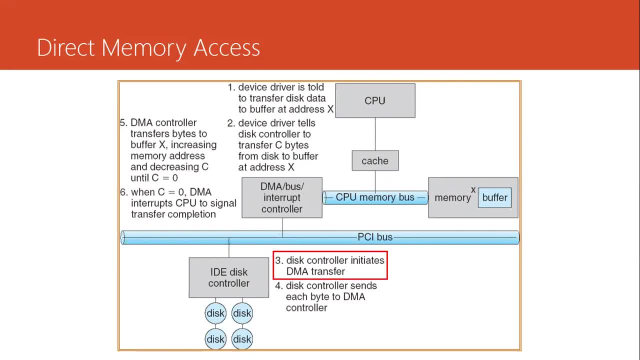 the number of required bytes. the disk controller then initiates the DMA transfer. after it moves the head of the disk to the proper place, the disk controller sends each byte to the DMA controller. the data passes through the disk controller and through the DMA controller and into the. 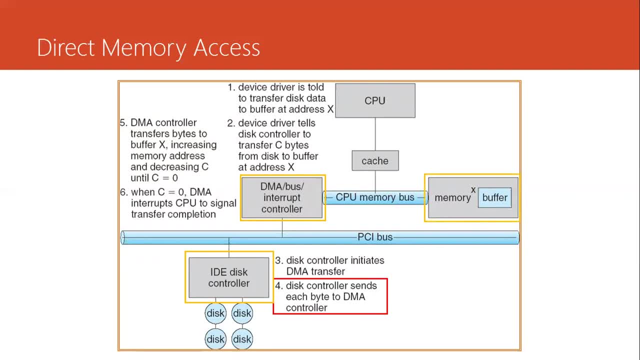 memory without the processor even being involved. the disk is doing the transfer automatically by incrementing the buffer address location and decrementing the C counter. C is the amount of bytes requested, and when they're transferring the data to the processor, the transfer is done, C becomes zero. and when C becomes, 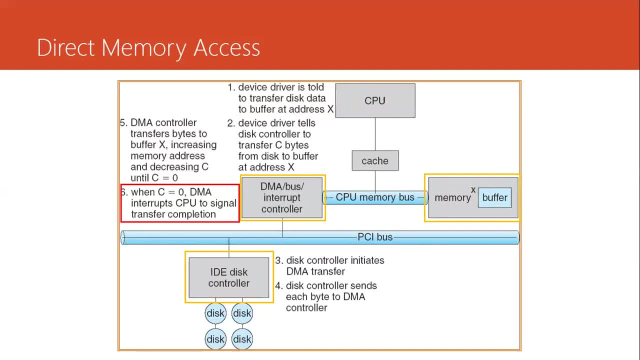 zero. the DMA interrupts the processor to signal it that the transfer of the required data is complete. so the processor has only set up the transfer and started to perform other activities while the data was being transferred and then can access the data from the DRAM. so the processor just let it go until the 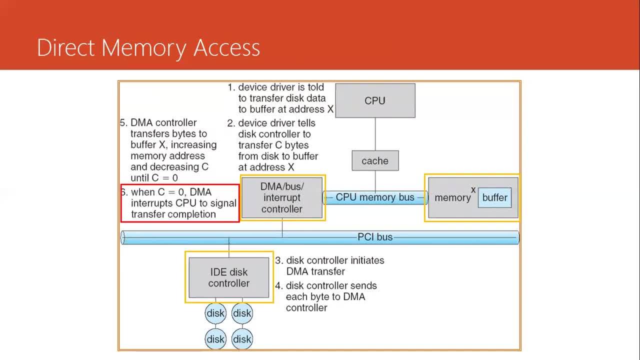 data is transferred and then the processor interrupts it when the transfer is complete, so this is one of the fastest modes of data transfer that actually existed from a very long time, as the processor resources were very scarce and requiring the processor to monitor and control the flow of data is a very 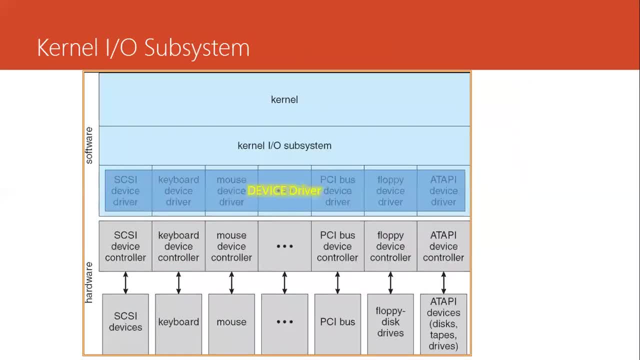 expensive procedure right. so far we have understood the concept and requirements of device drivers that knit together all those devices out there in the market that really don't work in the current market and the that really don't work in the current market and the that really don't work in the current market and the 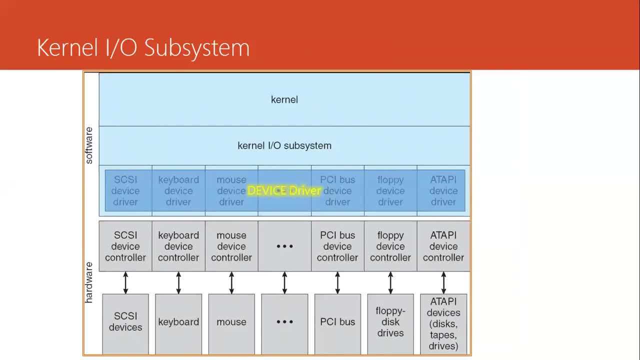 requires completely different interfaces based on their transmission speeds, predictable, unpredictable behavior, reliability factors and a whole range of operational parameters related to how they transfer their data. so let's take a brief look at the kernel structure for the IO system. the kernel tries to hide all these different structures and ways of interfacing them, so a typical 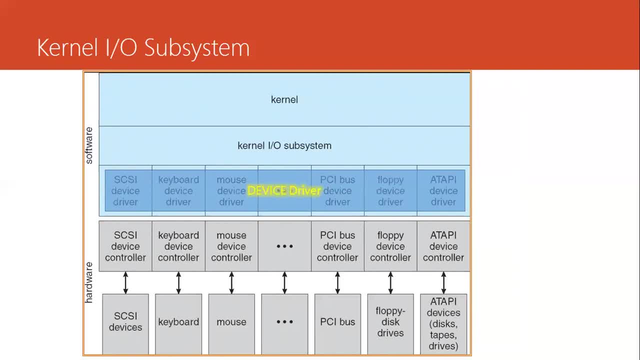 structure of the kernel has a kernel IO subsystem that presents a standard set of interfaces to the kernel and to the user as well. so this is a kind of a similar abstraction model that we studied earlier relating to the computational structures that divided the application load into chunks of 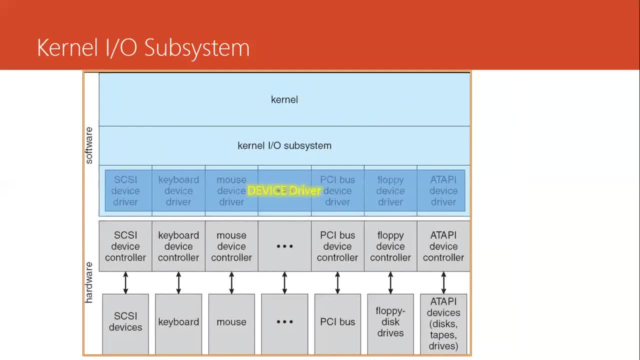 processing that actually worked on top of each other, with only interfaces to the upper and lower levels, and each level transformed the results or the inputs from the upper layer into something that served as the input to the lower levels, until the problem could be run on electrons. so we studied that computational model in one. 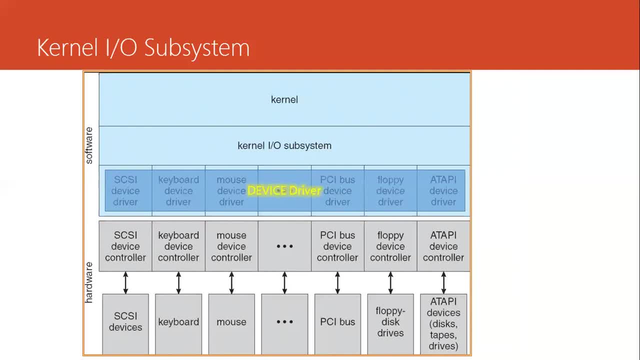 of our lectures. ok, so in that model we saw that the more you go closer to the hardware into lower levels, the more you need to know about the hardware. if you are working in c plus plus versus c, then c language is closer to the hardware versus assembly, which is even. 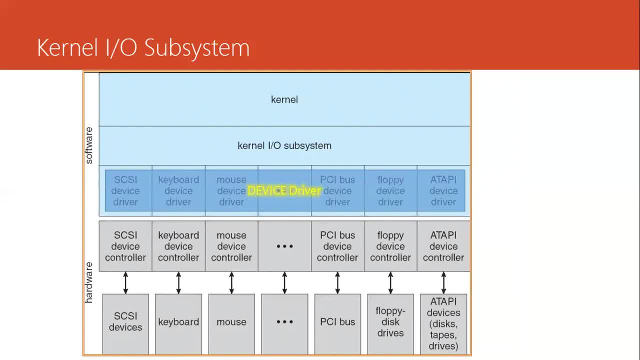 more close to the hardware and- and you need to know a lot about hardware while programming in assembly language right. similarly, we have one abstraction model here that has its own requirements of the breakdown of the workload. so the closer you go to the hardware, the more you need to know. 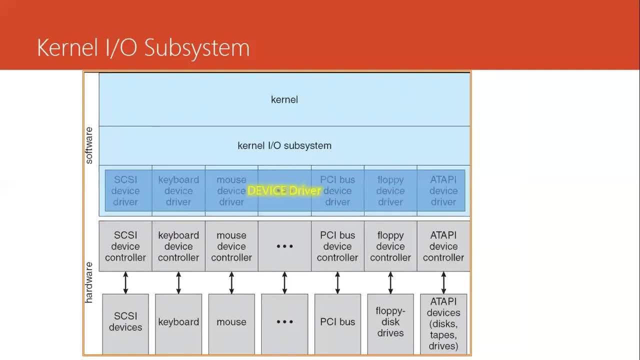 about the hardware devices and all the background information that we have studied until this point. at the top of the user program level, uh, sitting on the kernel that provides user IO libraries, the studioh and iostreamh, which provides standard io operations such as the printf, scanf and cout and cm system, calls: 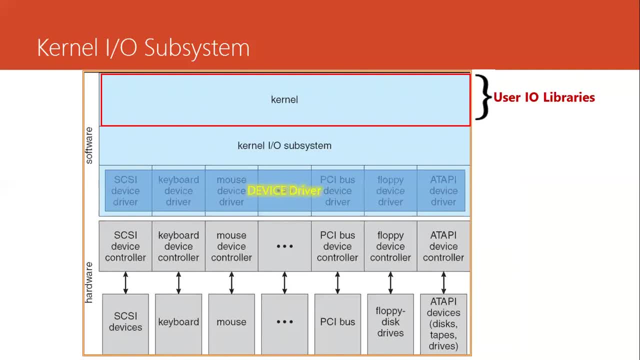 the user only needs to familiarize with the parameters of these functions without knowing much about the hardware. and using and using these high level system libraries, the user invokes the kernel i o subsystem, which is actually part of the kernel that interfaces the user with the device controller. 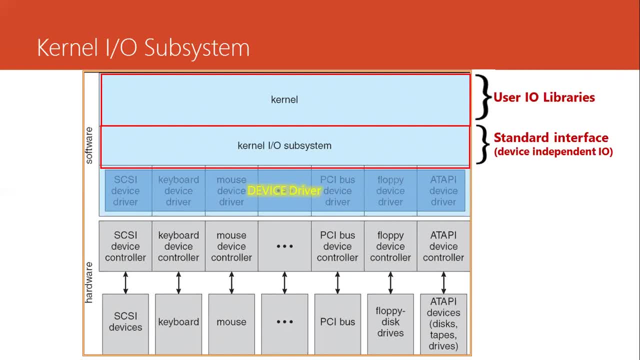 kernel ios systems are standard interfaces: device independent i o libraries. the kernel i o subsystem interfaces the user with the device controller. the kernel ios subsystem interfaces device controllers through the device drivers right. so this is the place where the device driver actually fits in, so it is a part of the kernel. 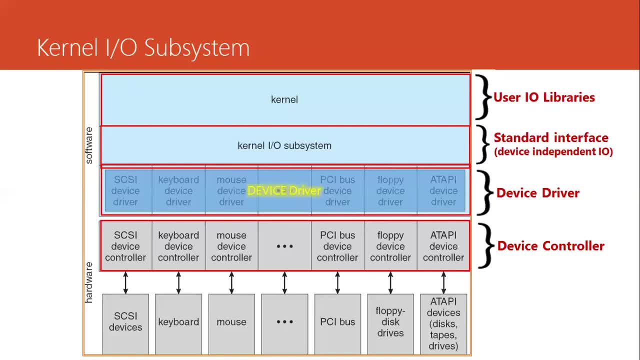 subsystem. so you can imagine how much of device hardware you need to know while writing code in the device driver level. yeah and finally, this is the actual hardware device. every one of the device drivers you load that is going to talk to a device has to meet a certain interface criteria so that you can use. 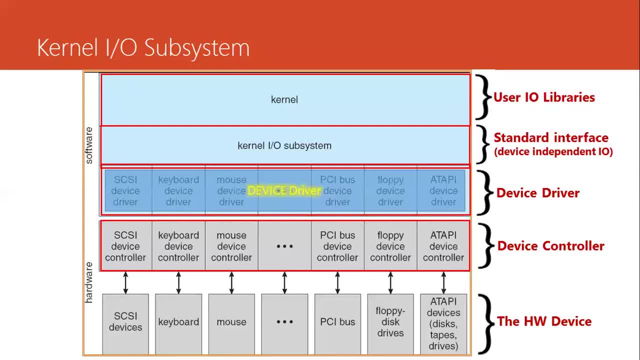 that device, no matter how it works. for example, you might have a SCSI device that talks to a disk drive. you might have a PCIe that talks to a disk drive. you have a floppy that talks to a disk drive. you have a USB that talks to a disk drive. a whole range of possibilities right in all of those. 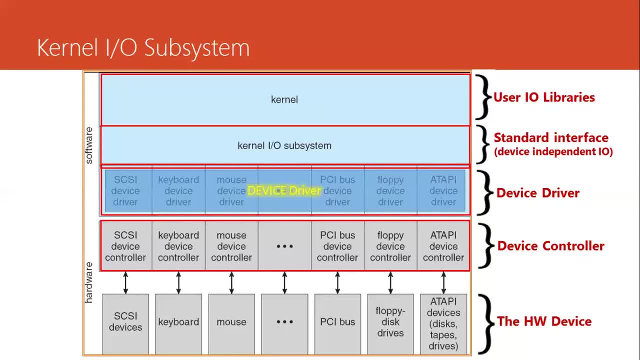 cases, even though every device is very different. you can use a file browse on them. you can use a file browse on your USB, copy something and go to your disk and paste it on your disk and that really works. so good device. so the final thing you have to do is to open up the machine and 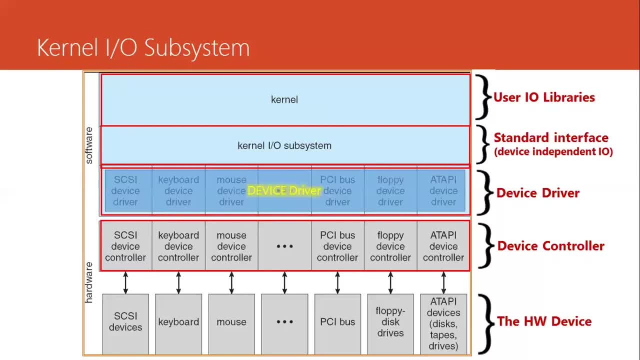 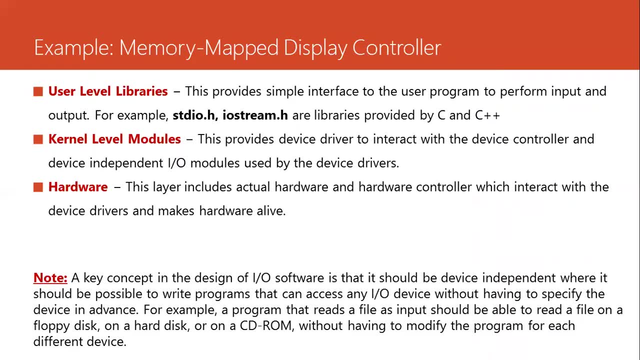 drivers could make a lot of difference in any computer system and sometimes when you update your drivers, all of a sudden your system starts to work faster. right as a recap from the last slide, we have the user level libraries. this provides simple interface to the user program to perform input and and output. 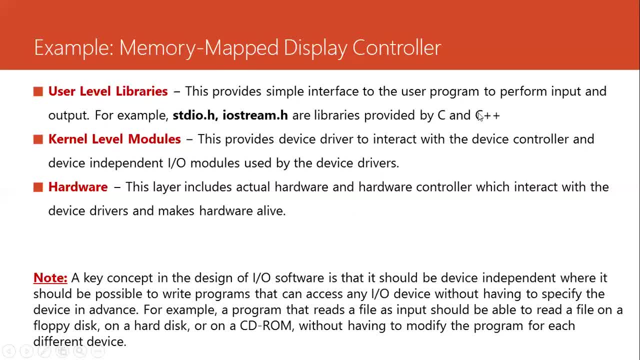 operations, for example the studio and iostream provided in the CC plus plus libraries. the kernel level modules. this month this provides device drivers to interact with the device controller and device independent IO modules used by the device driver. so this is basically the part of kernel IO subsystem and then 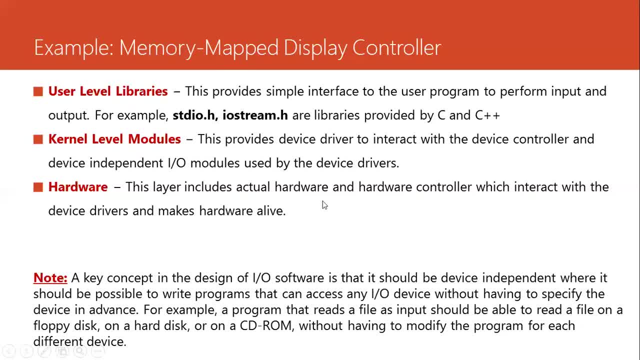 you have the actual hardware. this layer includes actual hardware and the hardware controller which interact with the device drivers and makes hardware alive. so just please note: a key concept in the design of our software is that it should be designed to be able to work with the hardware and the hardware controller. 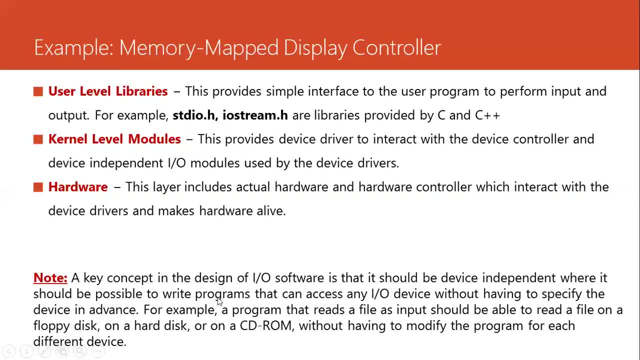 should be device independent, where it should be possible to write programs that can access any other device without having to specify the device in advance. for example, a program that reads a file as input should be able to read a file on a floppy disk, on a hard disk or on a CD ROM without having to modify the 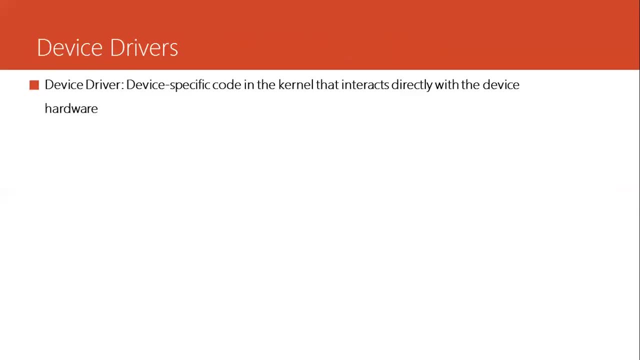 program for each different device. okay, so device driver or device specific code in the kernel that interacts directly with the device hardware and, as we already know that it supports a standard to the operating system, right, the important thing is that from the top, the same kernel, iOS system. 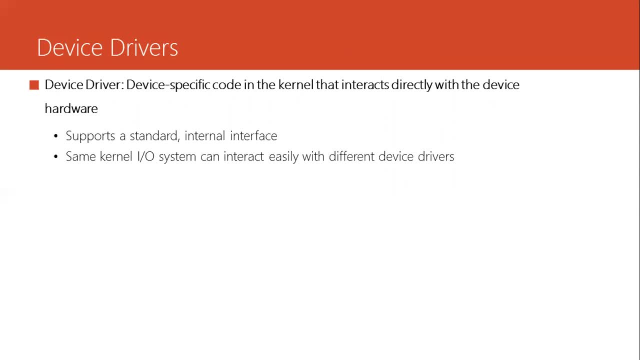 can interact easily with different device drivers and special device specific configuration is supported with the system called used in Unix and Linux. it is abbreviation of input output control and it is a system call for device specific input output operations and other operations which cannot be expressed by regular system calls. it. 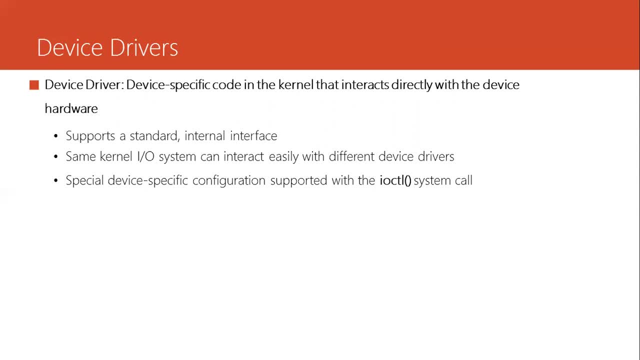 takes a parameter specifying a request code. the effect of a call depends completely on a request code. request codes are often defined by a device specific. okay, for instance, as CD ROM device driver can instruct a physical device to eject a disk for by providing an I octal request. 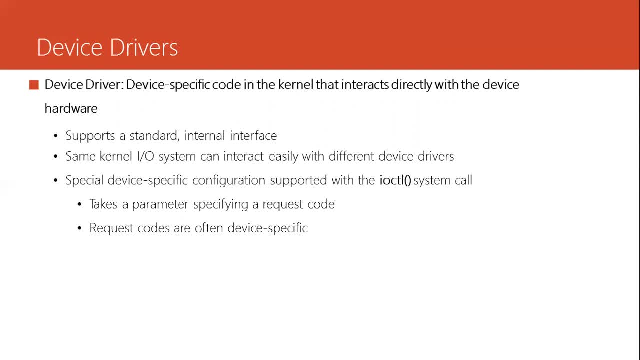 code to do that. if you go to the main pages of the I octal system call in Wikipedia, you will notice a broad collection that uses the I octal system. call for performing a wide variety of operations because different I octal work for different devices, so for 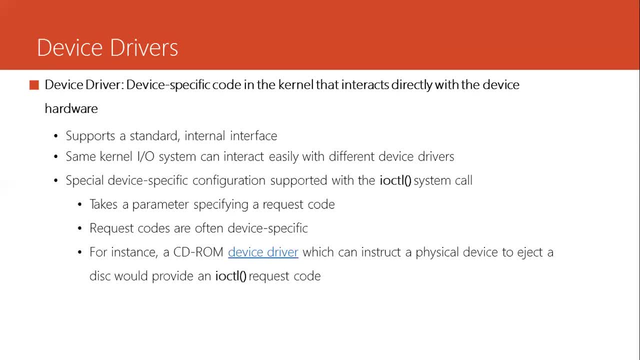 example, if you are dealing with a blocking interface, you would require the services of the I octal to to do actually change it to a non blocking interface. so you would first open that device and then you would do an I octal on that device to turn it into a non blocking. 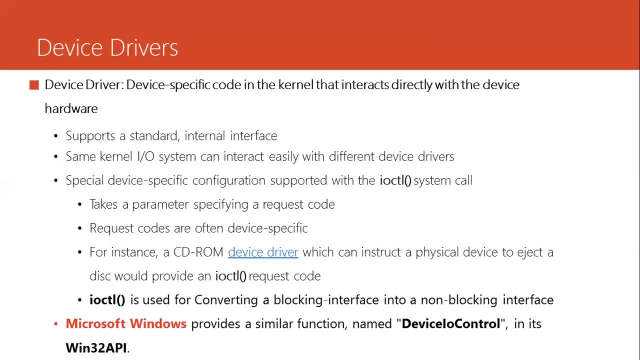 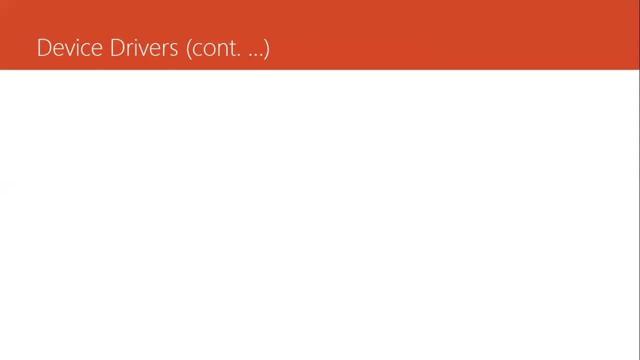 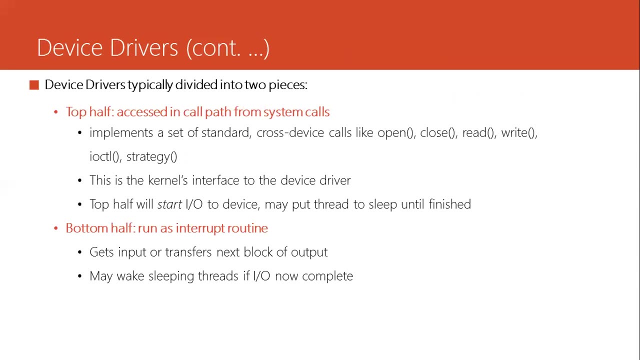 interface and you would see that this is a device. the control is can be disposed of through an I octal system. now you can see that device driver and then it can turn itself into an I octal. so it is basically a typical I octal system. so the application features it a lot of different things, like the: 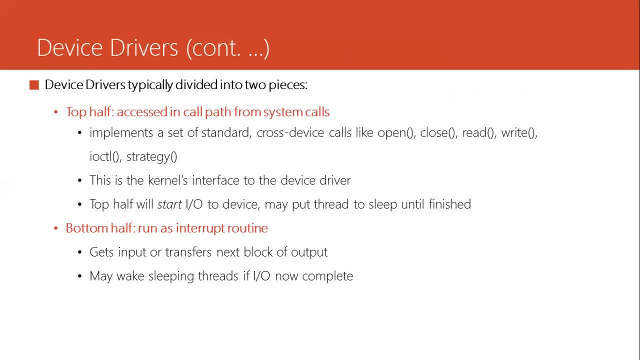 system calls is basically two parts to it. the Microsoft Windows provides a a lot like your system calls, like open call, close read, write I, octal strategy, etc. so some of these are not things that you give to the user directly, but they are mostly standard interfaces and the top up is the part that starts the I. 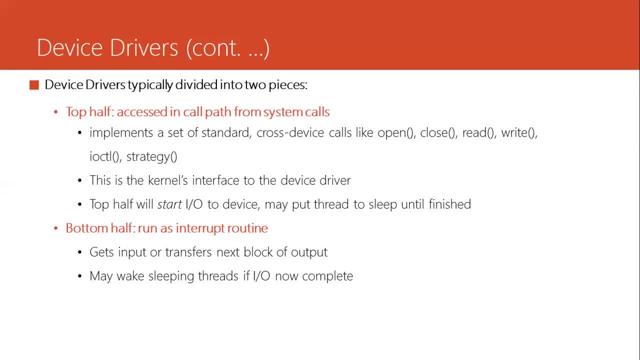 operations and then put a process to sleep until the results are completed. so the top half is the part that knows about the process. the bottom half runs at interrupt level and it does not know about a process from a thread. all it's doing is that it only takes notifications that an operation is. 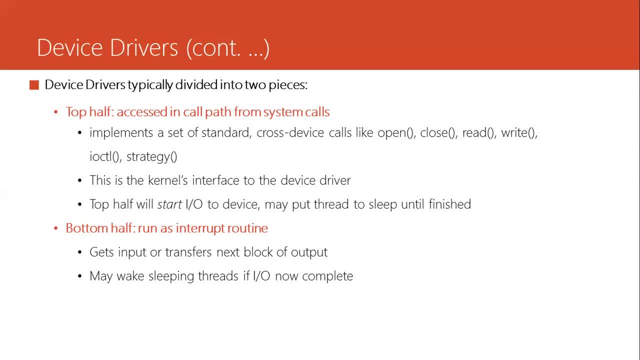 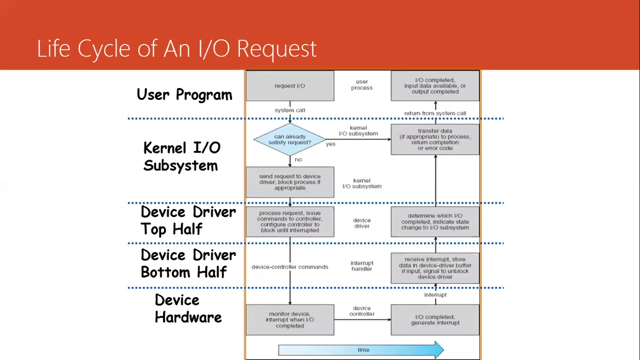 finished. so the bottom half works at a very simplistic form and it's only running in the interrupt level and has its own stack and all okay. so, in a more simplistic words, the bottom have basically responds to the top half and signals it when certain I operations are completed and the top half then figures out what to do. this is the 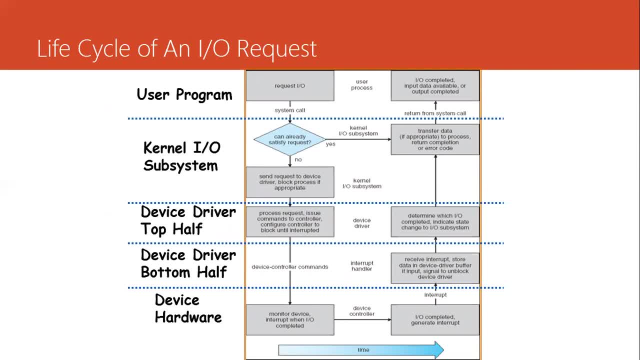 lifecycle of an IO request. the user requests kernel IO subsystem and, in a non-blocking case, if the device has a non-blocking interface. so it is possible that we are never going to go further, further than this control block right, because, as we know, that in a non-blocking 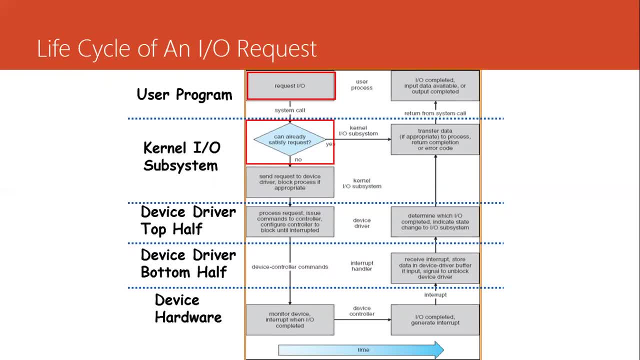 interface. we can always get back immediately with whatever data we have at hand and and maybe the system needed 100 bytes but the kernel system returned only two. so the system might request the kernel again for the remaining bytes and it is possible that the data has been cached in some way and it get to whatever. 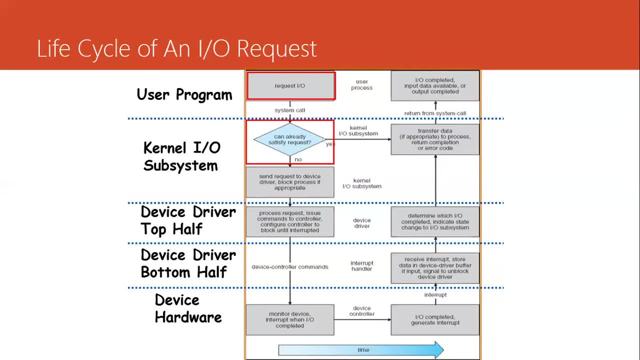 data is available me. however, in the case of a blocking device interface, the boredom IO subsystem might not satisfy the request, and in which case it sends the request down to the device job work and the top half of the device driver will put that process to sleep and it will start the 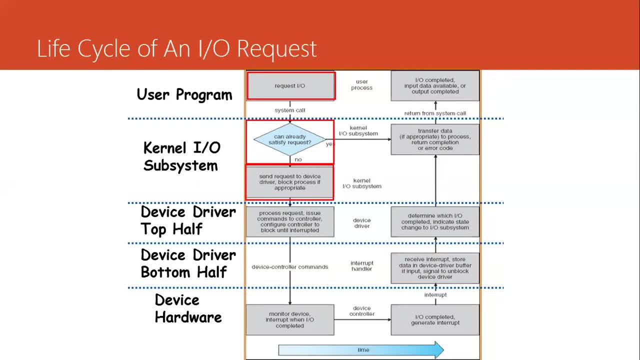 X's going so it. so it kind of tell the process that, since I don't have your data, so I kind of tell the process that, since I don't have your data, it starts up to 안에, so i might, which case, if the device sets up to sleepI might be able to turn off. let 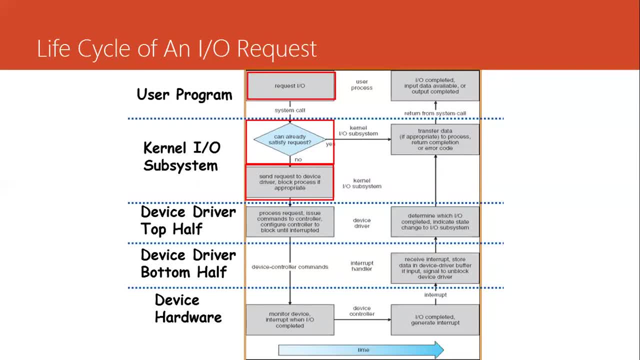 see, I am going to what I thought. thatErwin Airanti, You did that very well, but the cыв has to act immediately, the request getting to the device all the를 so. so we will put you to sleep and we will start moving, and later and later. 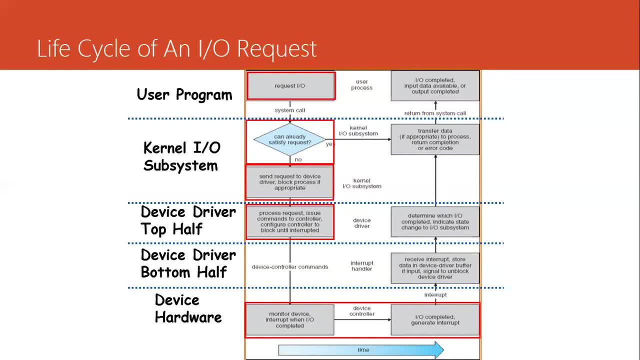 when the device is done, the data is stored in the device driver buffer and the bottom half checks the interrupt and signals the top half about some completion of IO and at that point the top up takes up the process and determines which IO is completed and transfer data back to the user and 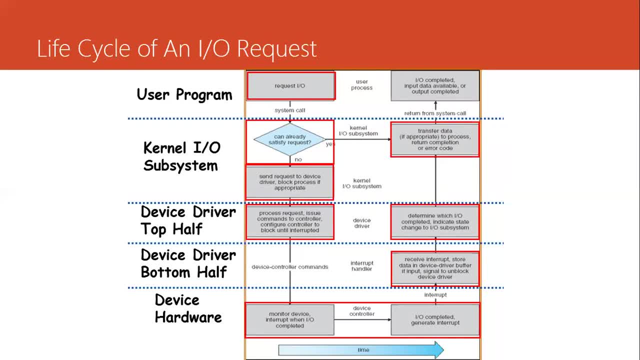 returns from the system call. so this is the kind of interaction between the top half and the bottom half of the device drivers. so clearly, if you are writing code for device drivers, you would have to adhere to a set of interfaces. writing device drivers is a very specialized skill that is out of the scope of these. 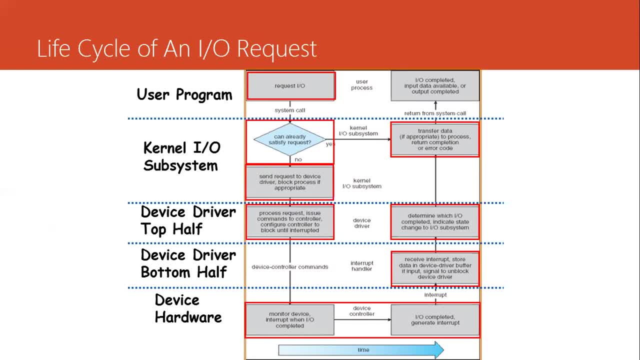 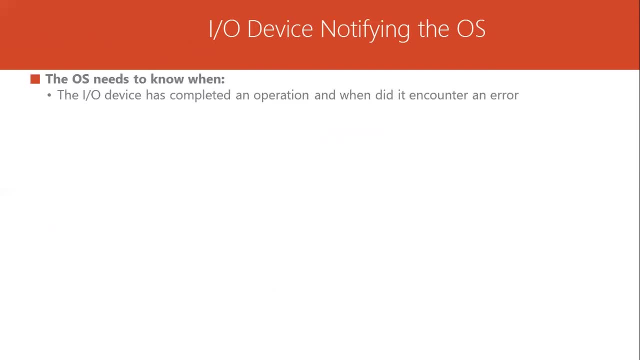 series of lectures now. now, how does the operating system know that the device is ready? so this is ultimately: the IO is completed. so how does the OS know that the device is ready? so the operating system has issued a command to the IO device, either by a special instruction or 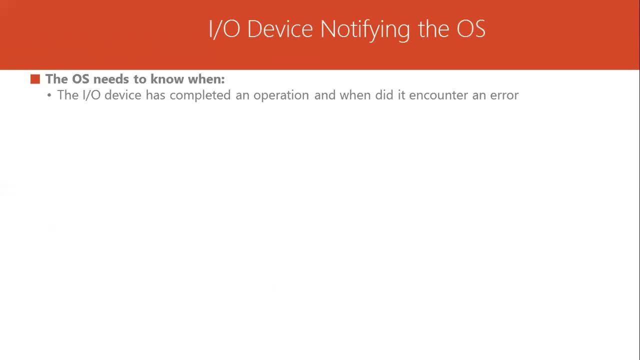 you to a location in the IO address space, and the operating system needs to be notified when the IO device has completed an operation and when did it encounter an error or when did it encounter an error? this can be accomplished in two different ways, either through IO interrupt or or. 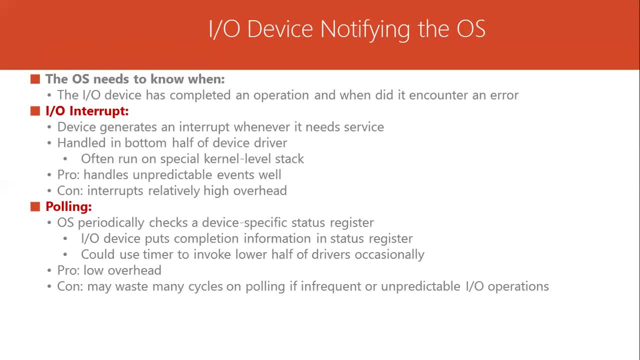 through polling. both of the methods have their own pros and cons. the downside of the interrupt based method is its relative high overhead, whereas the polling method wastes a lot of cycles on watching over infrequent or unpredictable events related to some device. interrupt are great for working with unpredictable. 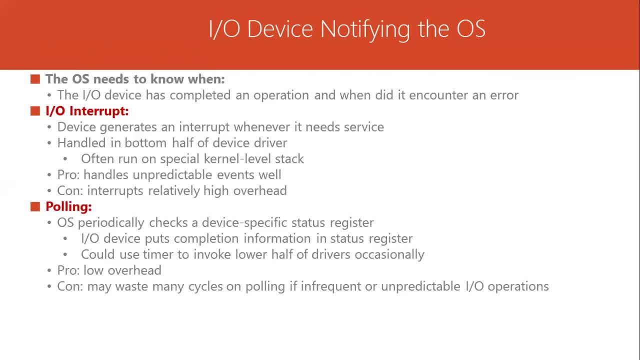 devices and you never waste time on on polling. so, in short, if the device use an interrupt to notify the processor of an event, this type of IO is known as the interrupt driven- and if the device has a status register that the software must periodically check, this type of IO is said to be based on polling method actual. 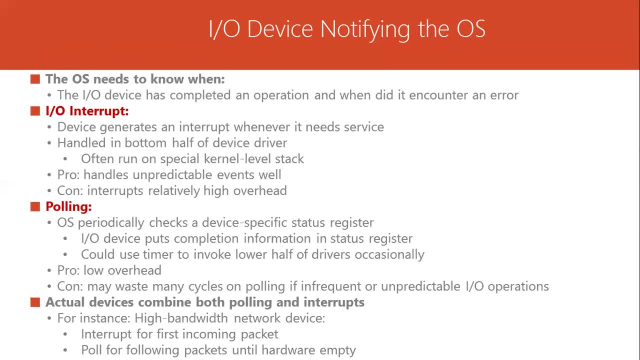 devices combine both of the worlds, for example, high bandwidth network devices. as we know that the packets are received randomly, as they might take different paths and, depending on the protocol, the network might also recent any lost packet right. if you were to interrupt on every packet coming coming in, you would simply overwhelm most. 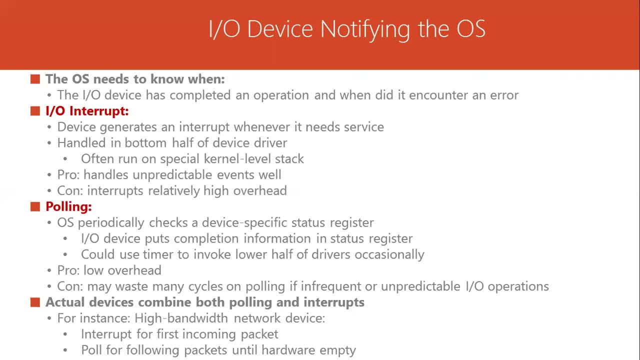 processors because there is not enough processing power to handle all the saving and restoring of registers and dealing with the interrupts. so what usually happens is that the first packet causes an interrupt once it gets it in an interrupt handler. the other packets are pulled until it empties out the 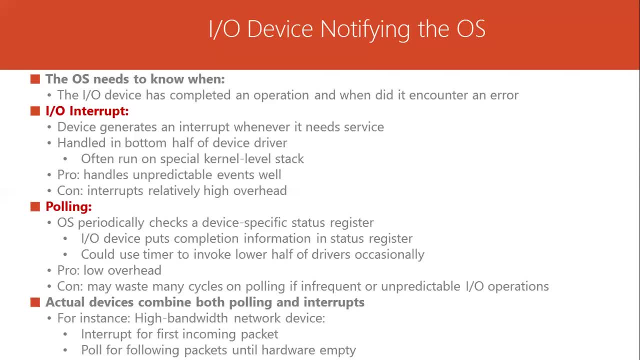 network card and then it re-enables the, the interrupts and gets back to the non polling state. so it's a combination of interrupts and polling to get an interrupt in the first packet and poll for the rest right. so while polling you are either using an iron section where you use in a in out instructions to read or write into the. 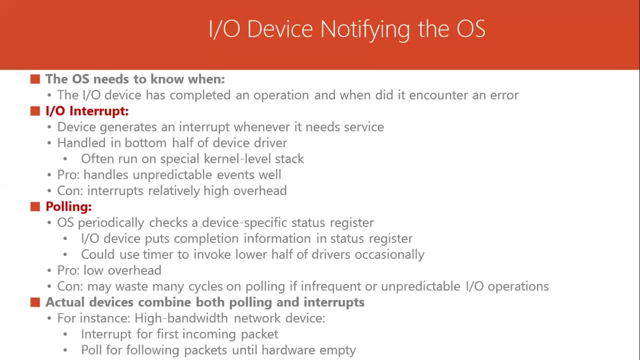 memory or, if you are, if you've got a memory map status register, so you are doing a load store operation in that IOS case. I hope that you got the basic introduction into some of the requirements of the IOS systems that are important to understand if in future you plan to write code for device drivers. we 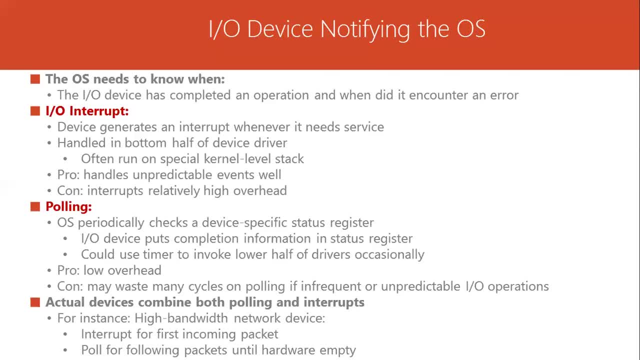 also looked into the different ways how a processor can access the registers on hardware device- you can access the registers on hardware device and how the data actually transfers between the device. and then we talked about the DMA interface, which is a very fast mode of data transfer. the DMA. 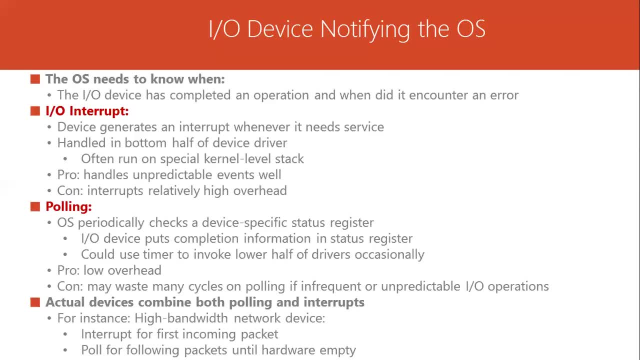 basically automates the process of transferring data between a device and the processor. the processor has to only initiate the transfer of the data, after which the processor goes to perform other activities and gets out of the loop. the device then gets ahead and transfer the data, and the DMA only interrupts the processor when the transfer is complete. then we